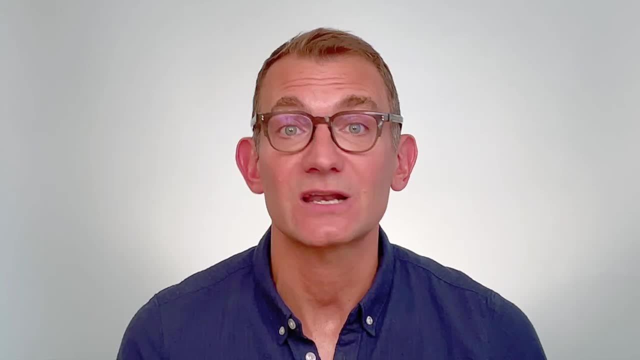 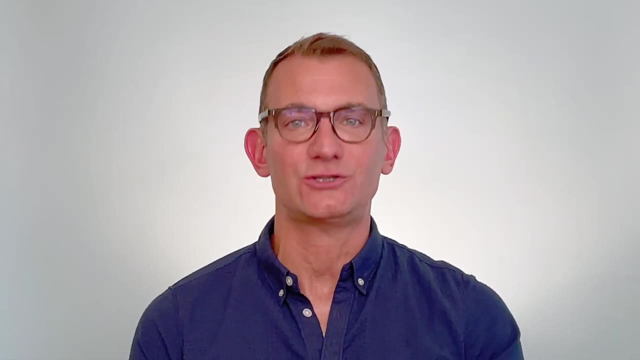 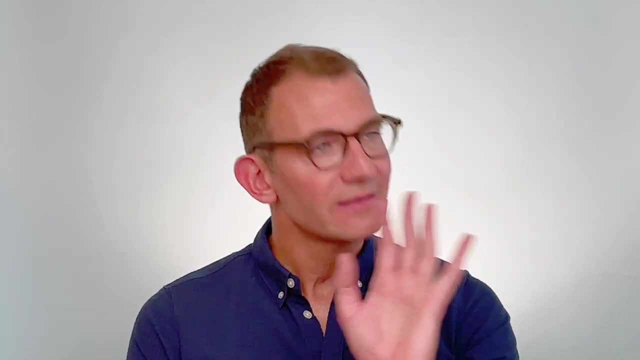 list plans. After four rigorous years of scientific study, we can confidently say that your biology degree will prepare you for more than medical school alone. You will graduate with plenty of highly coveted skills, including laboratory and research skills, And let's remember that employers in STEM fields need graduates that understand how. 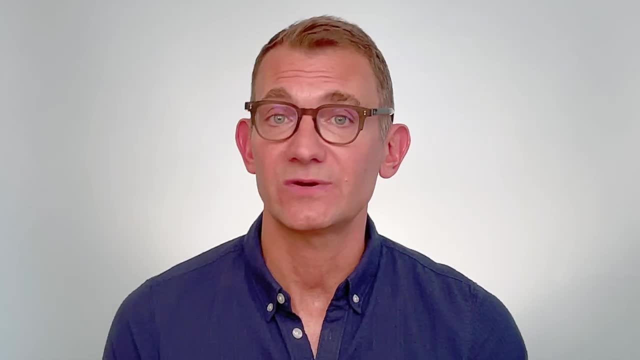 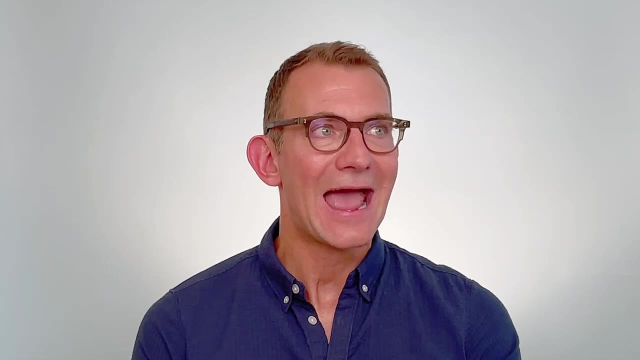 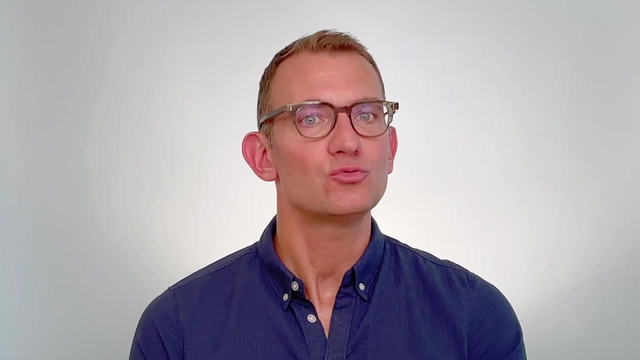 to define problems and design experiments and conduct research. Employers also look for folks with strong technical communication skills. Biology graduates can get paid to explain complex ideas to a non-technical audience. The ability to summarize scientific findings—with charts, with graphs and other visual aids—in 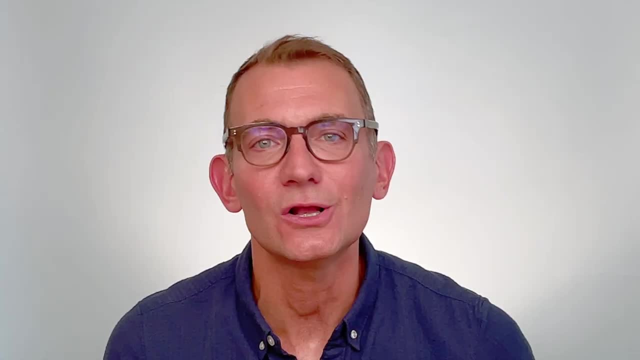 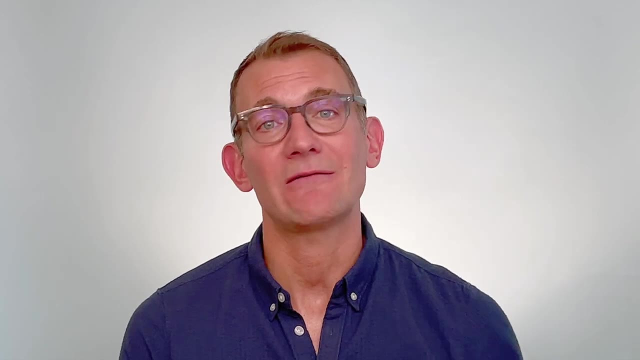 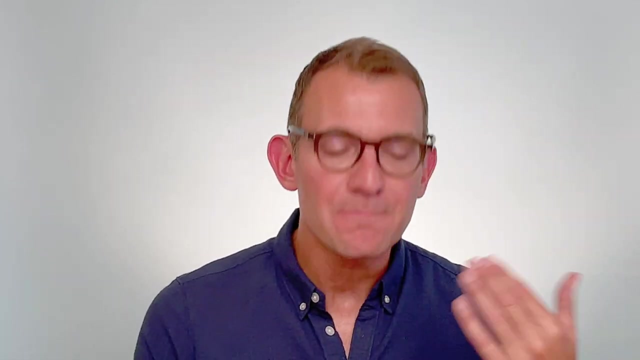 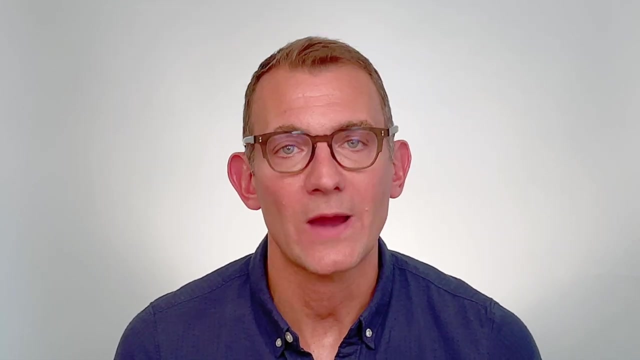 a way that non-science professionals cannot. That's why we're here today. You'll also develop advanced quantitative and data analysis skills, focused on your ability to use software and statistical tests to predict outcomes and model your research findings. Without a doubt, friends, they will prepare you for a wide range of careers in science. 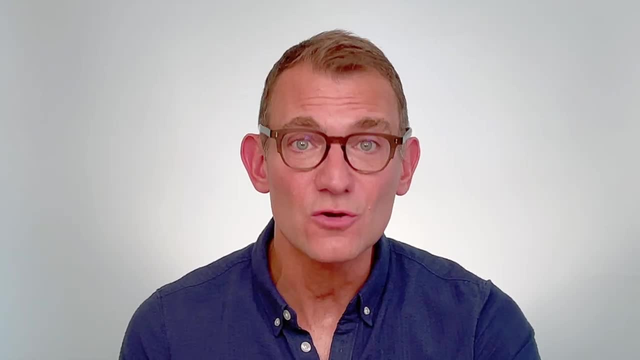 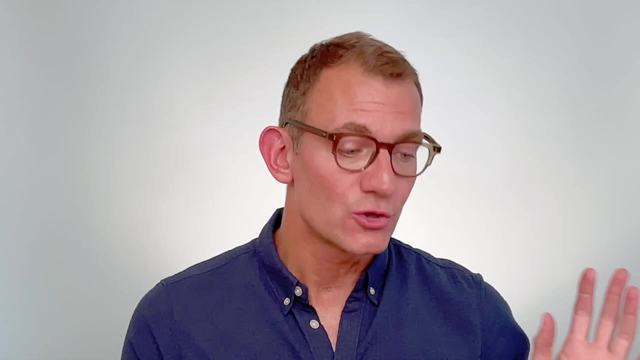 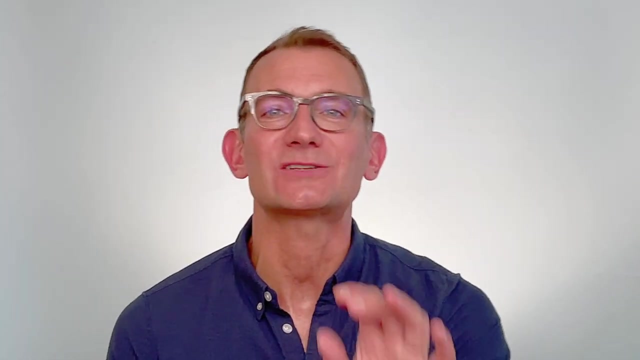 healthcare, business and government, And those are just to name a few. And that's not all. According to the US Bureau of Labor Statistics, STEM fields are expected to grow 8 percent by 2029.. That's over two times faster than all other occupations, which will grow at a measly 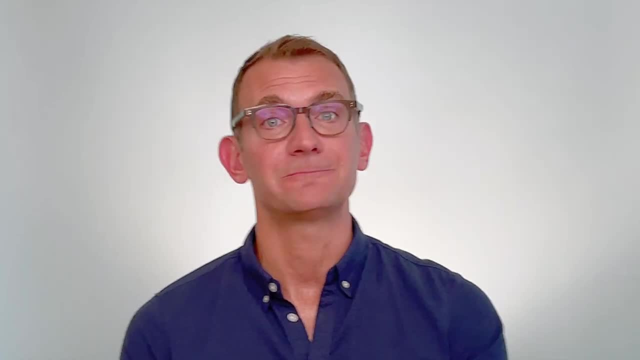 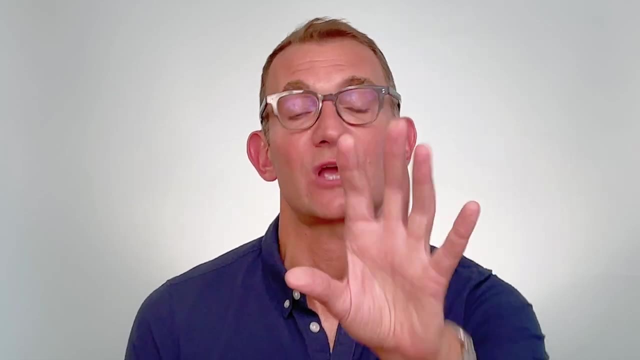 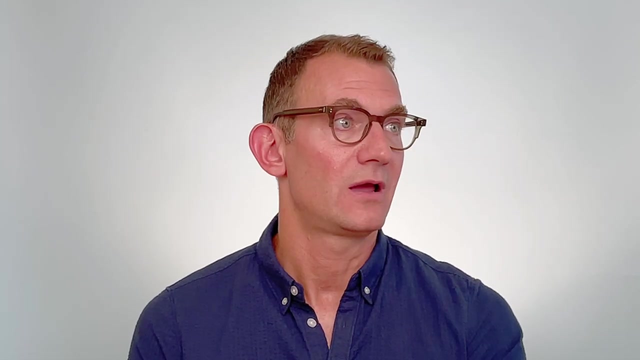 less than 4 percent in the next decade. This means that biology graduates can look forward to fast-growing and lucrative STEM careers, including positions such as biochemists designing studies for the development of new drugs and medications, environmental scientists, protecting the environment and identifying. 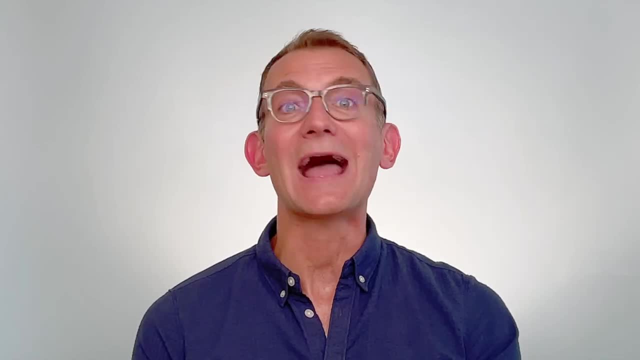 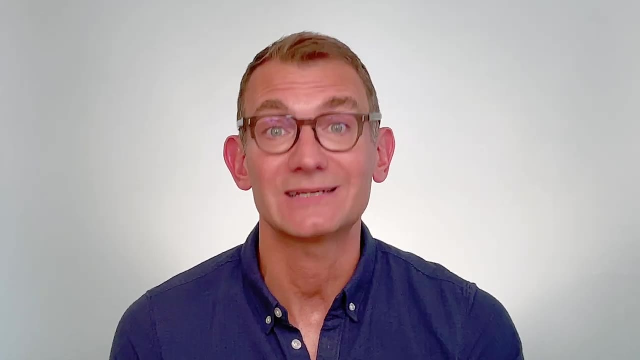 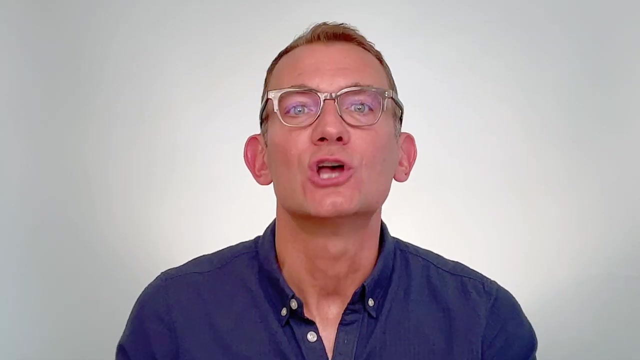 health hazards through scientific research. medical scientists discovering new approaches to treatment and disease prevention. biological technicians conducting tests and experiments in academic as well as medical labs at universities and hospitals. microbiologists studying some of the smallest lifeforms, including bacteria, algae and fungus. 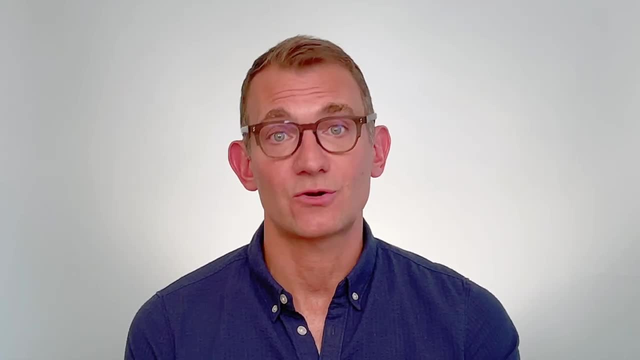 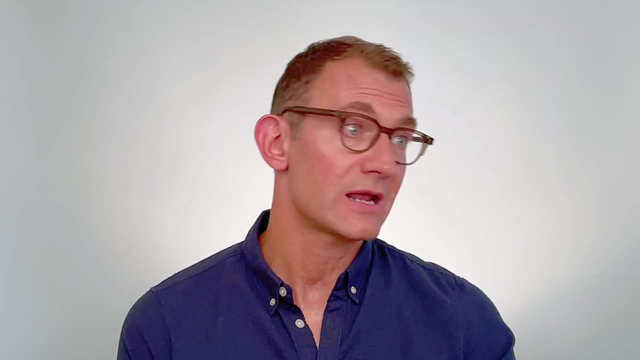 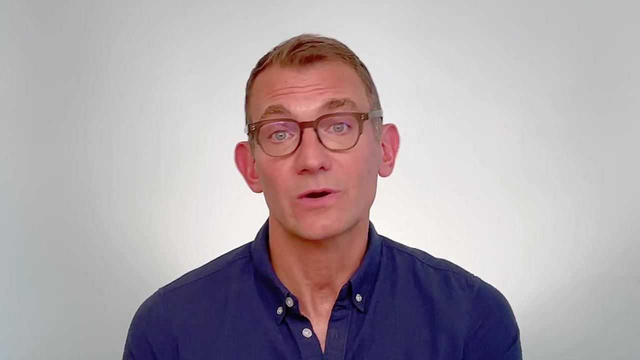 And folks that all said. many biology graduates opt out of traditional roles as scientists and technicians in favor of roles in sales, marketing, education, public policy and law. You'll find quite a number of biology graduates working as health policy analysts where you 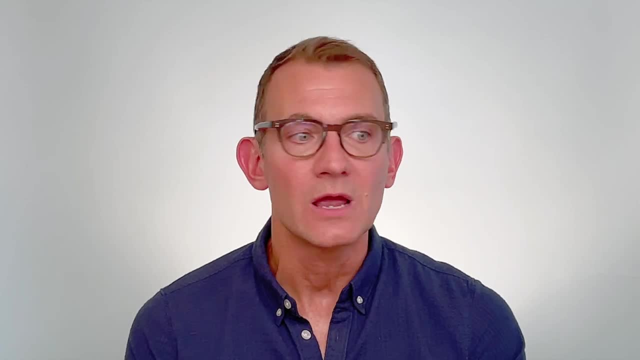 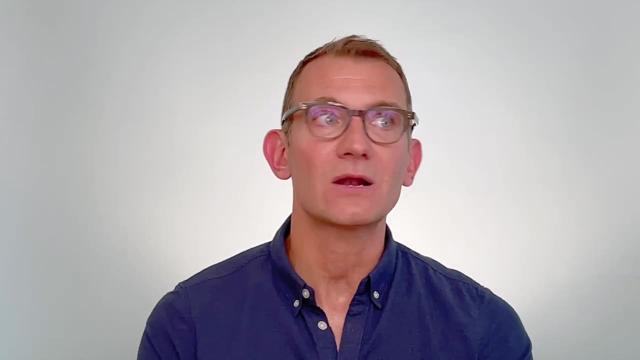 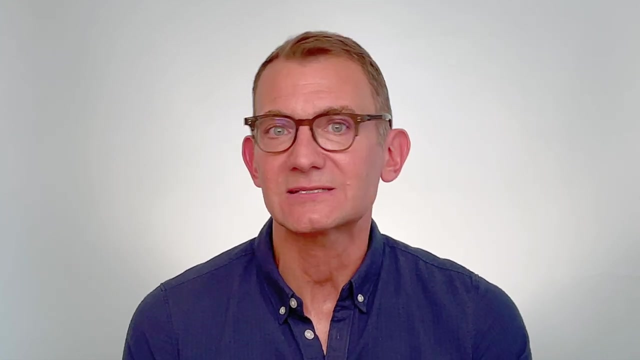 can find or chart a career in public policy, evaluating laws and government procedures, and in the field of science. In addition, this role will allow you to study programs related to health, medicine and the environment. A medical writer is an exceptional career for biology majors who love writing about. 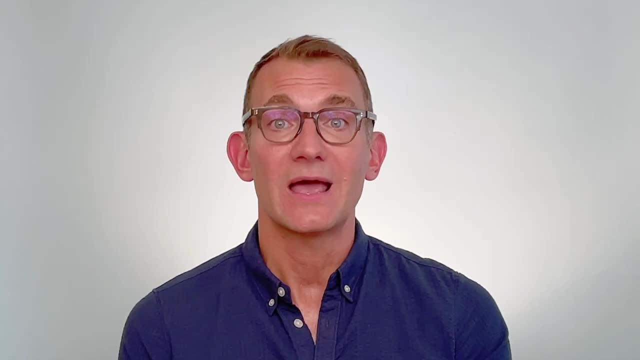 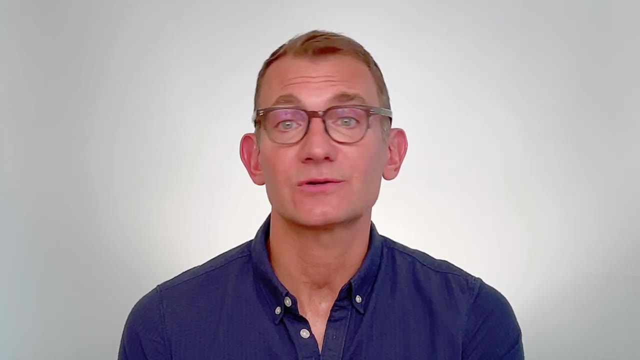 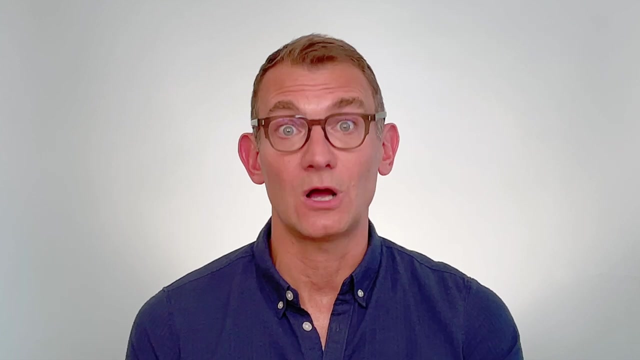 science. In this role, you'll be writing articles, technical manuals and technical documents related to healthcare and other scientific topics. A pharmaceutical sales representative. if you're interested in traveling for work, then this role will allow you, without question, to travel to doctors' offices and hospitals and other healthcare facilities. 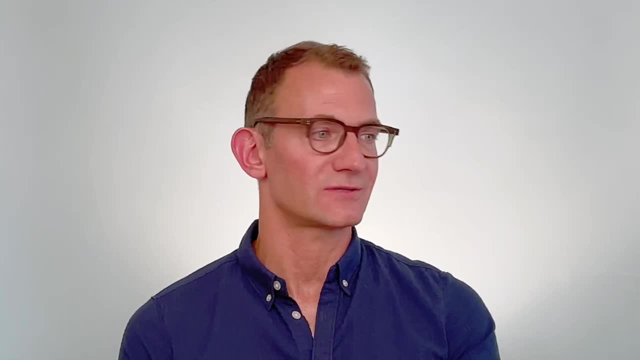 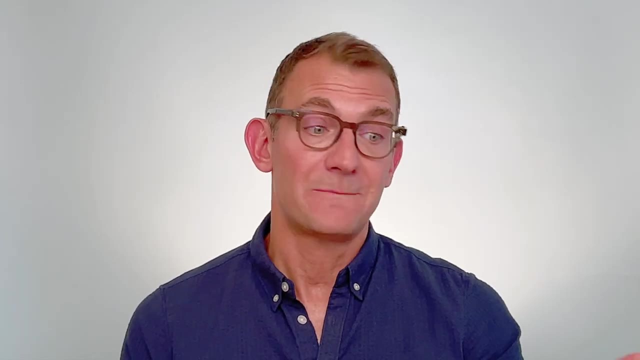 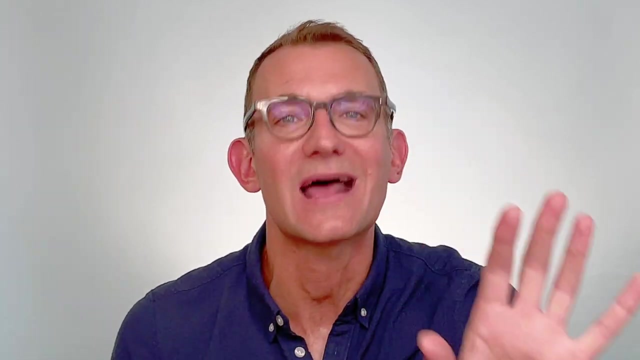 selling pharmaceutical products to medical professionals. Next, an attorney. You could use your biology degree as a lawyer to specialize in patents and intellectual property, medical malpractice or environmental law. Of course, this means that you'll eventually need to go to law school, but be that as it. 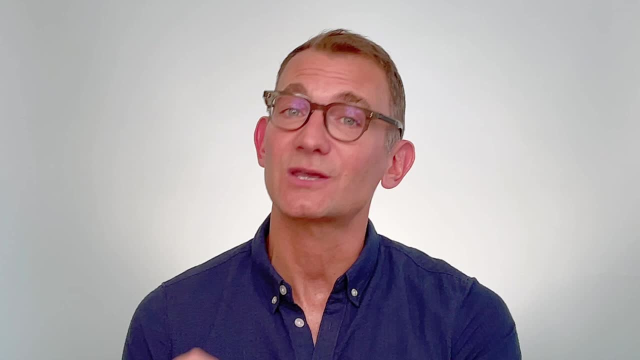 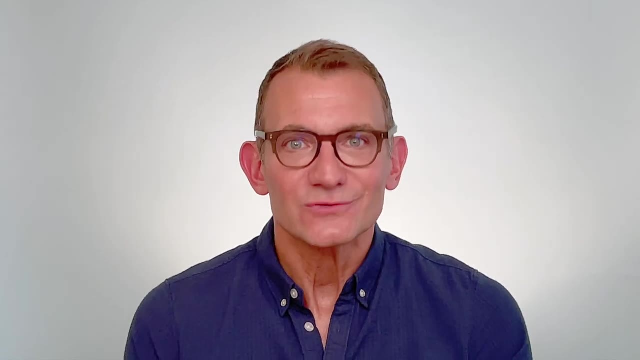 may, friends, suffice it to say that this list of possible occupations goes on and on. I'll hit just one more before we wrap up today's segment. A teacher: Folks, if you're interested in education, you should also consider a career as a biology. 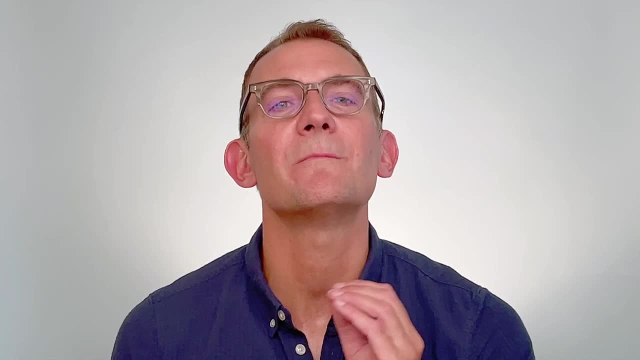 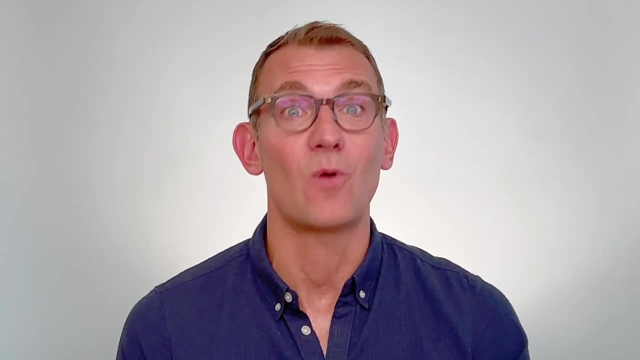 teacher. Again, friends, these are just a few of the many careers besides medical school available to you if you choose a major in biology. If you are a current or aspiring biology major, then leave us a comment and let us know what. 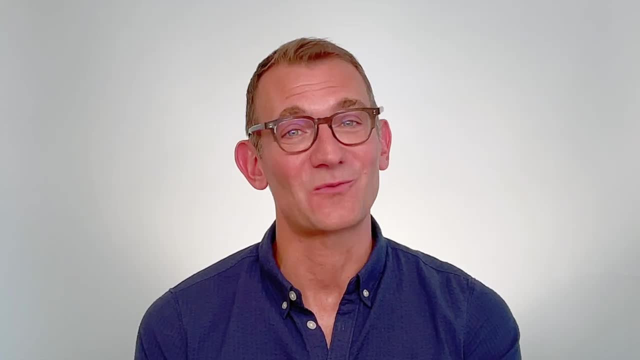 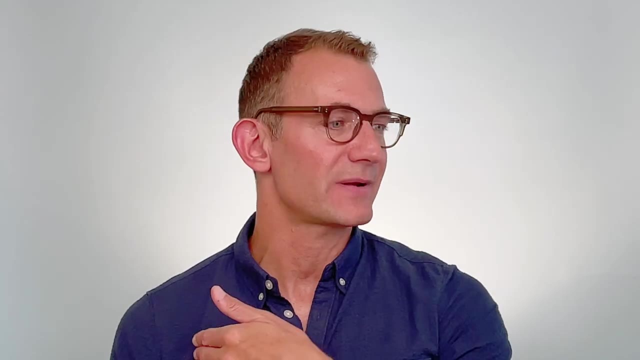 you plan to do with your biology degree. As always, thank you so much for watching these videos. Please subscribe. You can also subscribe to our channel, if you haven't already, for the latest and greatest updates about college test prep, career information, life skills and more. I'm Rob Franek, Editor-in-Chief here at The Prince Review. signing off, Be well.